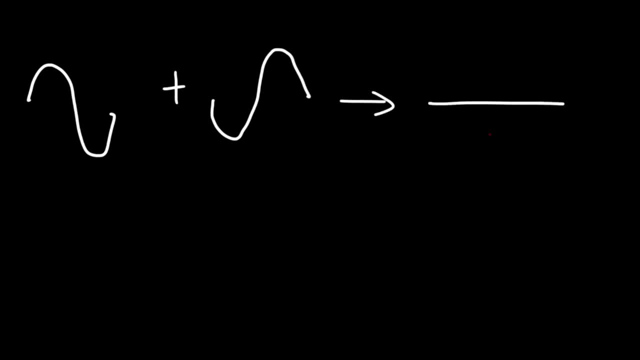 Well, destructive interference will occur and instead of getting a bond, you're going to get a node which is a region of zero electron density. So basically, the probability of finding an electron in this region is almost zero. Now, according to valence bond theory, a covalent bond is basically the sharing of electron density between two atoms as a result of the constructive interference of their atomic orbitals. 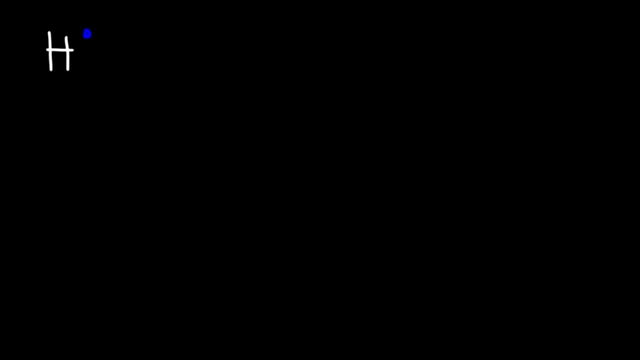 So let's consider hydrogen again. Hydrogen has one valence, electron, and the electron configuration of hydrogen is 1s1.. An s-orbital has a spherical shape, So this is going to be hydrogen with its spherical orbital. and let's react it with another hydrogen atom. 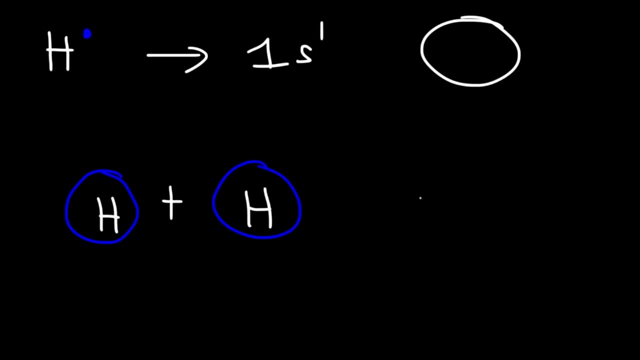 So when these two get together, their orbitals will overlap, and you're going to get something that looks like this, And so what we have in the middle is a covalent bond. Whenever two atomic orbitals overlap head-to-head, it's known as a sigma bond. 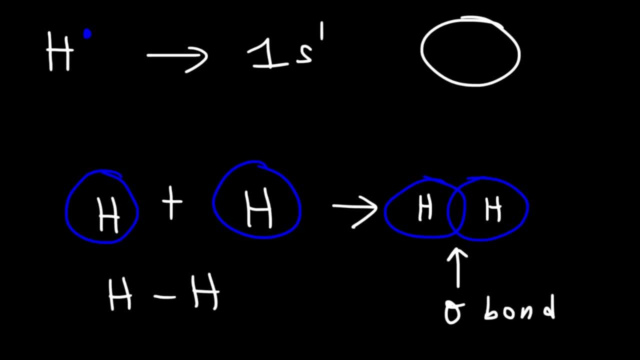 All single bonds are sigma bonds, so keep that in mind. Now, what about when carbon mixes with hydrogen? It mixes with hydrogen to create methane. In order to do this, carbon has to hybridize its atomic orbitals. It has to create hybrid atomic orbitals. 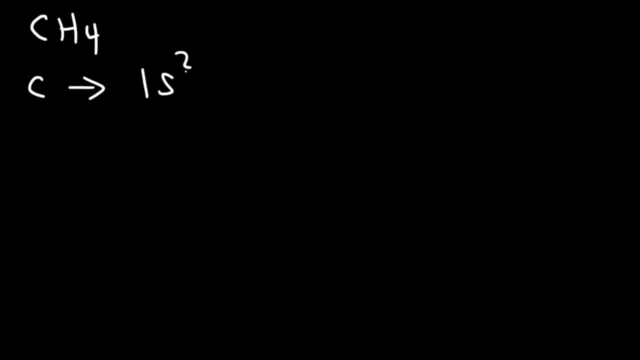 Now let's talk about the electron configuration of carbon. It's 1s2, 2s2, 2p2.. Carbon has a total of six electrons. Two of those electrons in the first energy level are core electrons and they don't participate in most chemical reactions. 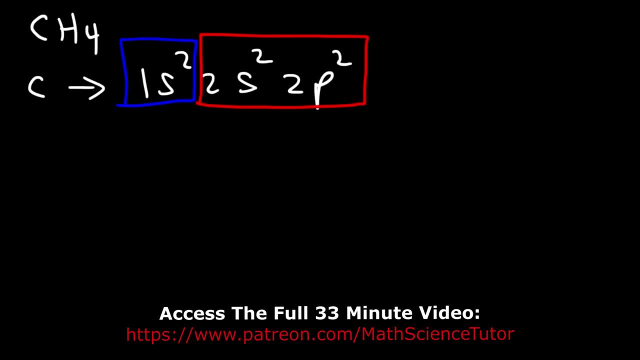 The other four in the highest energy level, are known as valence electrons, and the valence electrons do participate in chemical reactions. So let's draw an energy diagram for a free carbon atom. So we have the 1s level, the 2s level and the 2p sublevel. 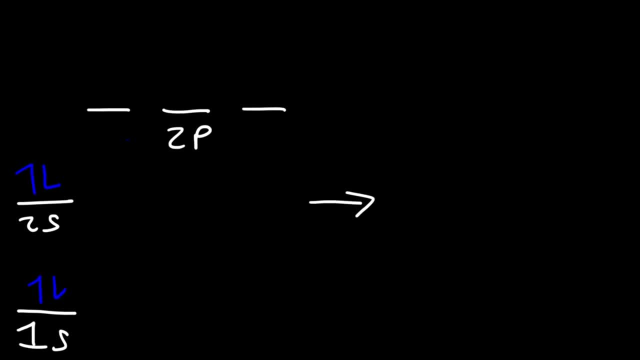 So we have two electrons in the 1s level, two in the 2s and two in the 2p sublevel sub-level. This is the ground state electron configuration for carbon In the excited state. an electron here could jump into this empty orbital if it's. 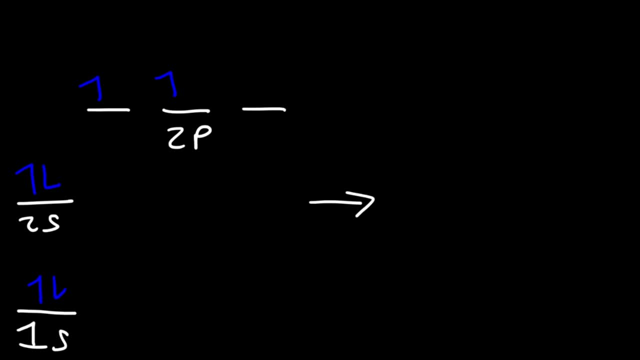 given energy. But right now we're going to just talk about the ground state electron configuration. So during hybridization, the 2s orbital and the three 2p orbitals, they're going to mix together to form a hybrid sp3 orbital. So 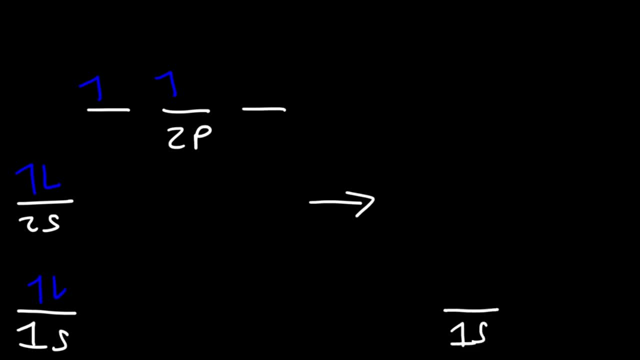 the 1s level is going to stay the same. Now we're mixing together four atomic orbitals, and so we're going to get four hybrid orbitals And they're going to be degenerate orbitals of the same energy. So if we mix an s and 3p orbitals, what? 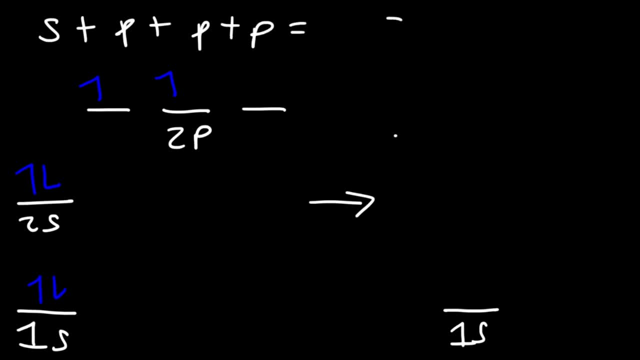 are we going to get? We're going to get a hybrid orbital called an sp3 orbital and because we mixed four atomic orbitals, we're going to get four sp3 orbitals. Now, what should be the energy level of an sp3 orbital? Should it be? 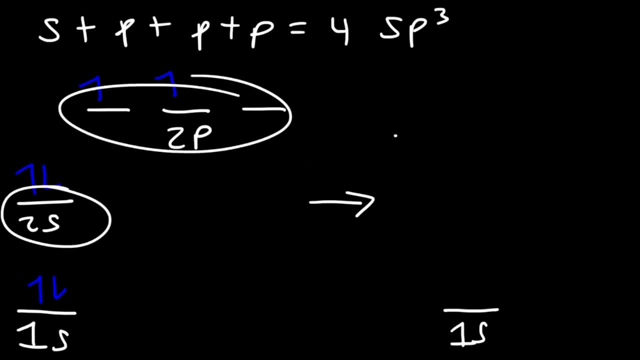 close to the 2s level or to the 2p level? What would you say? Because an sp3 orbital is produced from mixing 3p orbitals and 1s, it has more p character than s character. In fact, it has 25% s character, 75% p character. We have 1s. 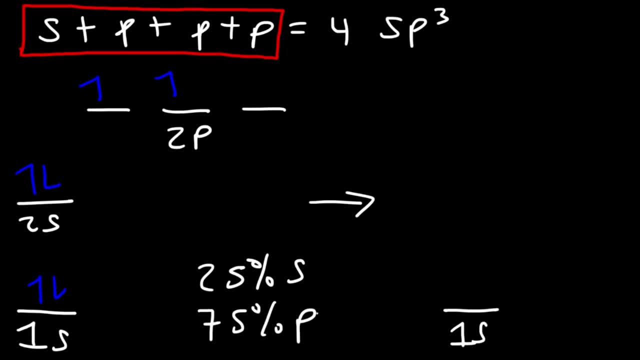 out of 4 atomic orbitals, so 1 fourth is 25%. We have 3p orbitals out of 4 atomic orbitals, so 3 fourths is 75%, And so, because it's mostly p, the energy level should be close to the 2p sub level, but a little bit lower than it. 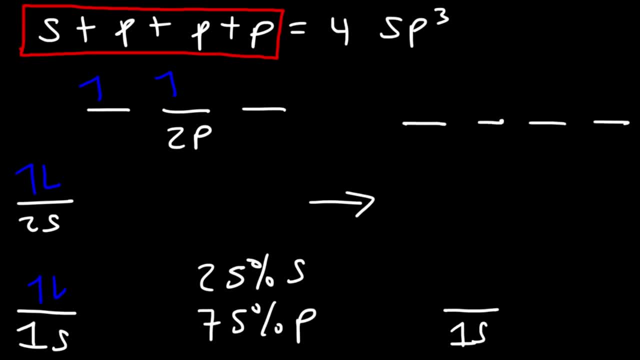 So we get four hybrid orbitals. These are known as degenerate orbitals because they have the same energy level. As a result, we're going to place all four electrons equally among those four orbitals of equal energy. So the 1s level. 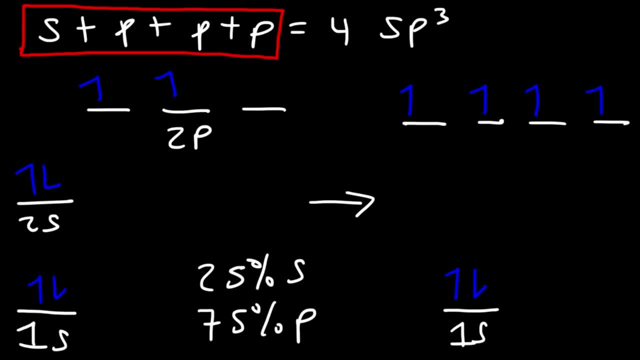 is unhybridized. it was unaffected, But these four atomic orbitals were hybridized into these three, These four sp3 hybrid orbitals. And hybridization is basically mixing. If you mix water with orange juice, you're going to get something. in the middle You can get a. 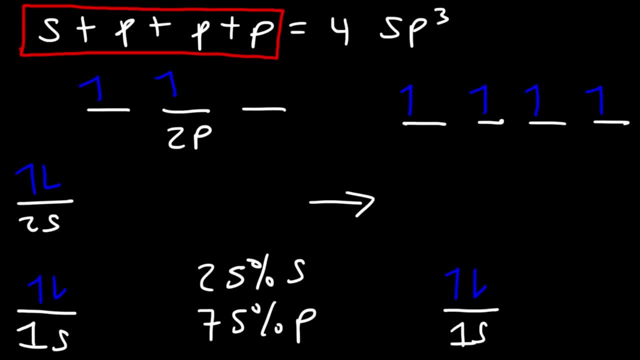 hybrid. Or let's say, if you mix orange juice and milk, you're going to get something in between, And that's what hybridization is: You're just mixing atomic orbitals. So if you mix s and p, you get something that's in between s and p. So these are the four. 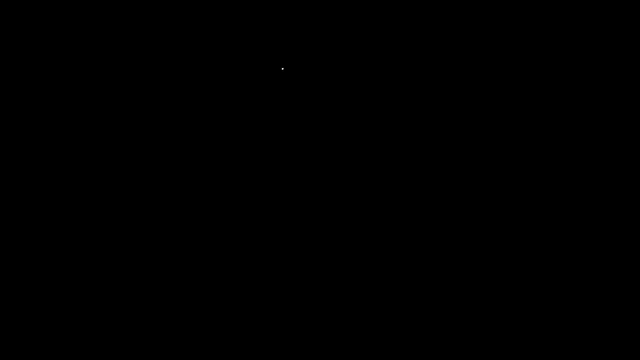 hybrid sp3 orbitals. Now let's go back to methane. Methane has four single bonds, and so it has four sigma bonds And, as we said before, the carbon in methane has four sp3 hybrid orbitals highlighted in red. And hydrogen can only form an s orbital because it 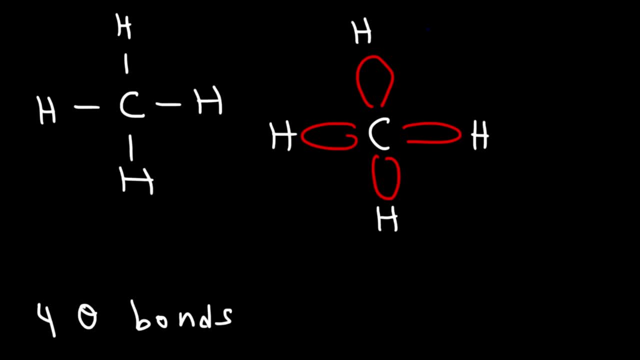 has one electron in its 1s sub level. So let's say, if you have a test question and it asks you: what is the hybridization of the central carbon atom? The hybridization of carbon is sp3.. Now how can we describe the hydrogen orbital? We can say it's simply s, And so 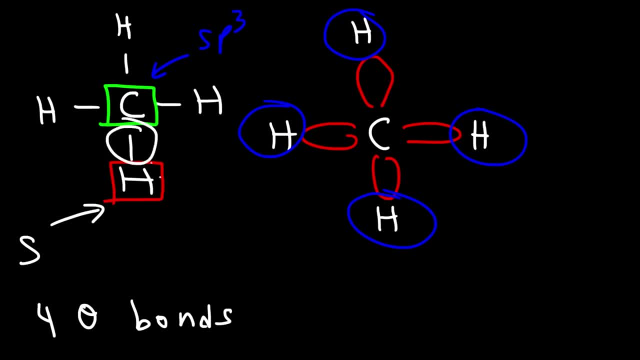 if we want to describe the bond that connects carbon hydrogen, we could say it's a hybrid of s and sp3.. Those orbitals in red are sp3 hybridized And hydrogen is simply an s orbital. So when you mix an s orbital with an sp3 orbital, you could say it's a hybrid of s. 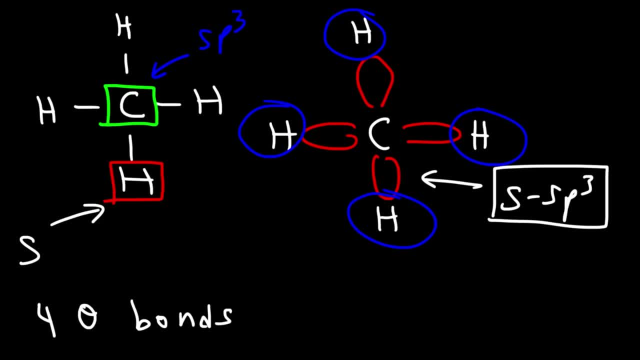 sp3.. So that's how you can describe the hybridization of the bond, And so anytime you have an overlap of atomic orbitals, You're going to have a sigma bond. So this whole thing is one sigma bond, This is another. 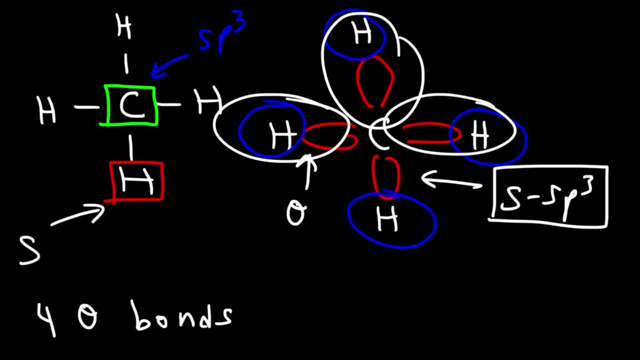 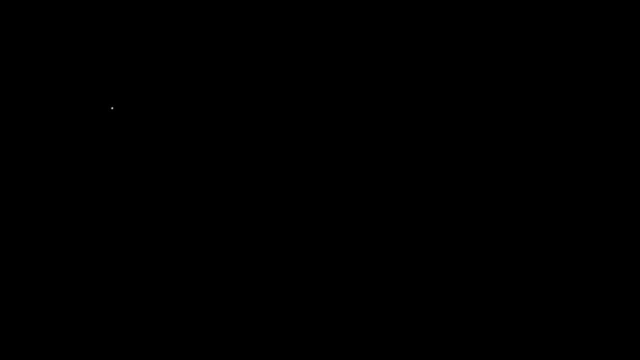 And so methane has four sigma bonds, or four single bonds, or four covalent bonds. You could describe it any of those three ways. Now let's talk about ethane C2H6.. How many sigma bonds are in ethane?